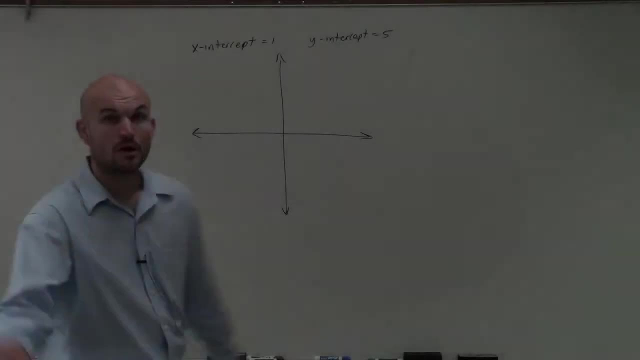 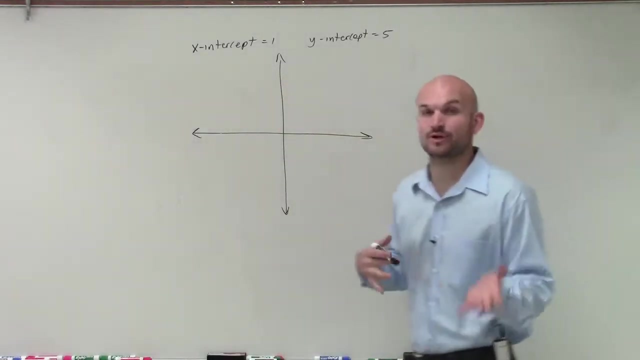 Welcome. So what I'm going to do is show you how to graph this linear equation when given the two intercepts. Now, it's important to understand when graphing, especially using intercepts, is what exactly do the intercepts mean and what are we graphing on? So this 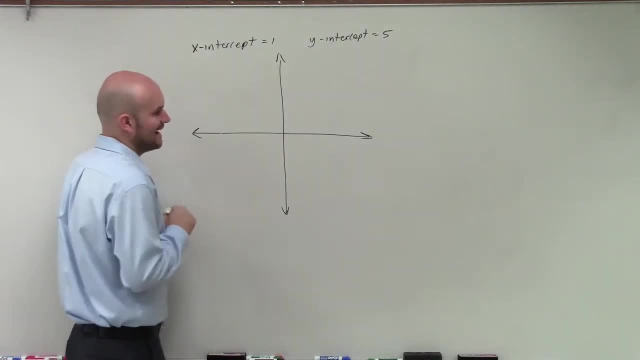 is what we call a coordinate grid, And what this grid includes is what we call the x-axis and the y-axis. Now, on the x and y-axis, what we have is, you know, just like- if you're kind of like number line- we have units that we break them apart And you can really break. 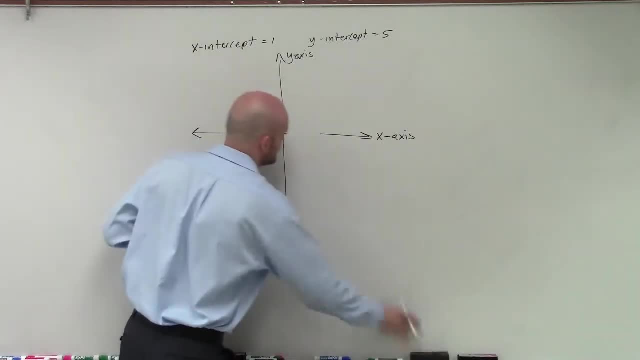 these apart on any way that you want to. It's all going to depend on a lot of problems are going to be different. I'm going to make these a little bit wider. So 1,, 2,, 3,, 4, 5.. So in. 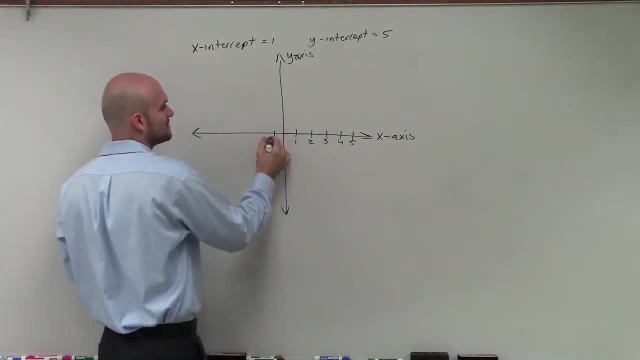 the positive direction, it's going to be positive, And then going over to the left, which would be the negative direction, And that's for the negative values of x. Now, what they mean is what these values- negative and positive, they're pretty much meaning. a distance from what we could say is this: 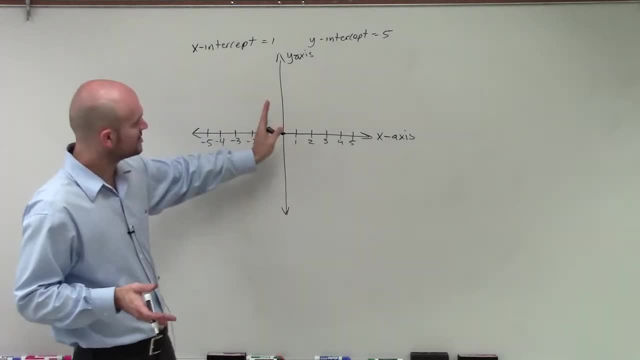 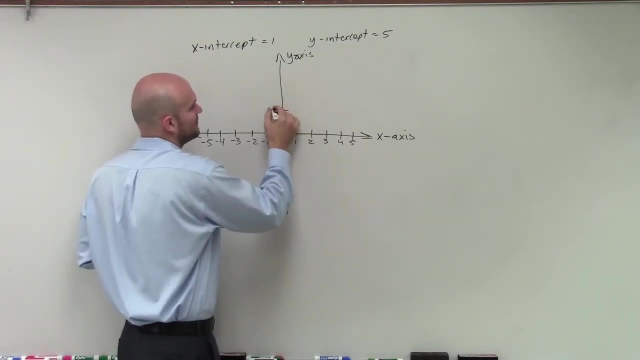 point which we call the origin. And we call it the origin because that's also where the x and the y-axis intersect. So for the y-axis, when we go up that's positive, And when we go down that's negative. 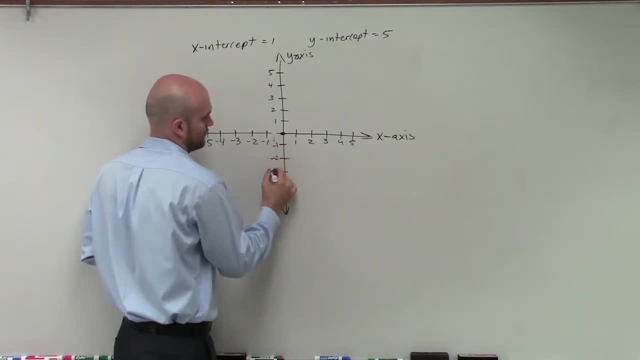 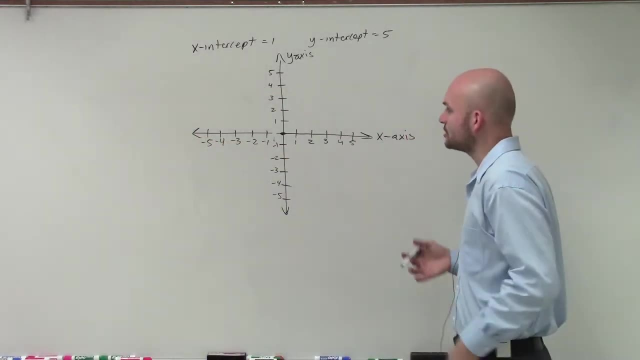 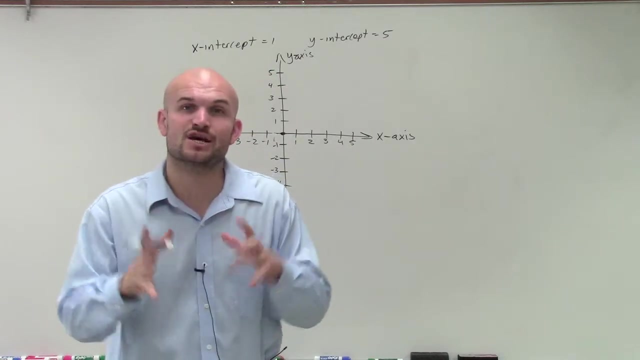 Okay. So I'm given two sets of information. I'm given the x-intercept and the y-intercept. So when we're talking about the x and y-intercept, that means those are the values, or at that x and y-intercept, that's where a point crosses each axis. So what I'm saying is the x-intercept. 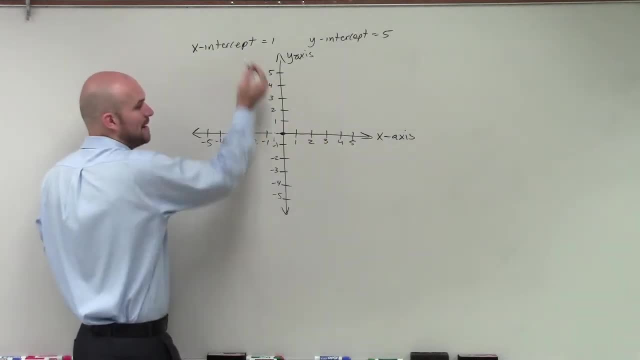 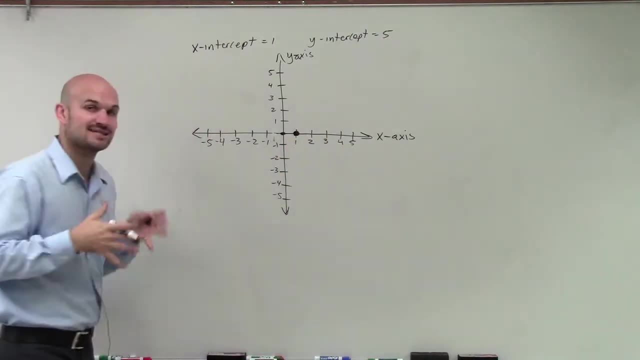 equals 1.. Well, since it's positive, it's going to be to the right, And that means the graph is going to cross when my x value is going to equal 1.. So I'm going to make a nice big point because that's going to be a solution to our linear 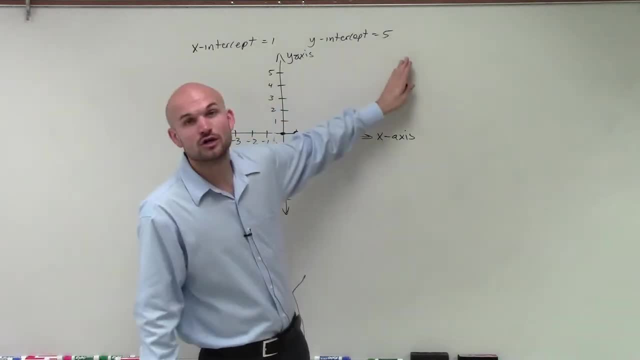 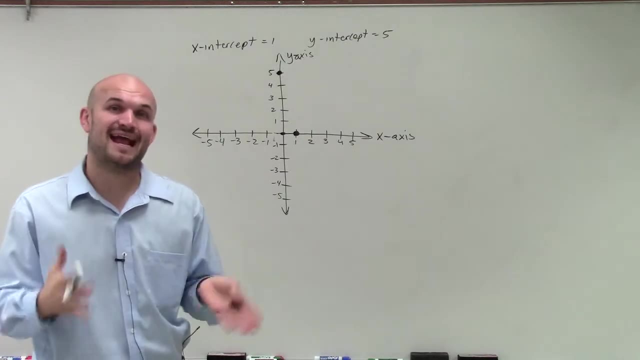 equation. Then it says the y-intercept is at 5.. So that's going to be positive 5.. So therefore that's gonna be my y-intercept. So now that I've found the x and the y-intercept to graph.